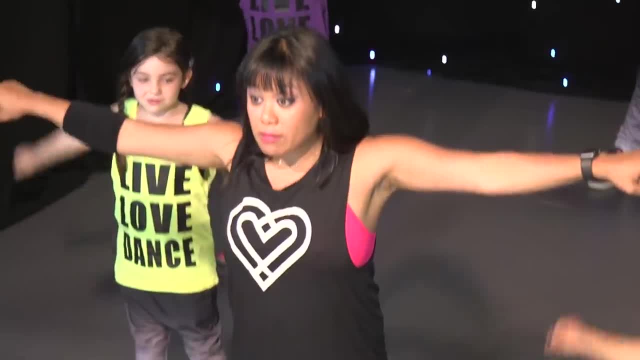 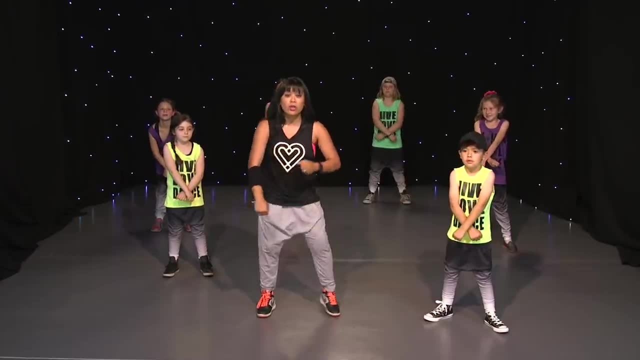 So cool, We call it airplane arms. Let's do the arms first. You're going to open those arms, Open airplane. Then you're going to cross them in front. Cross, open cross. You're going to take your right hand in the air and you're going to punch it: Punch, punch, punch. 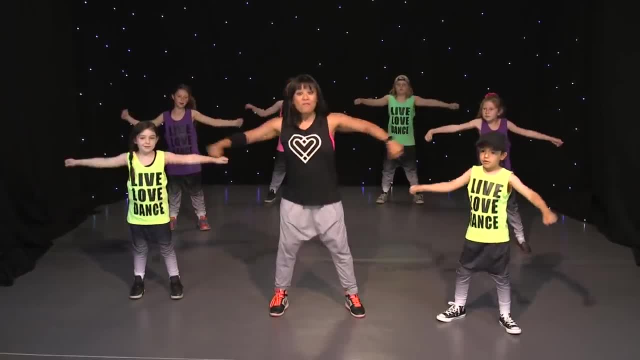 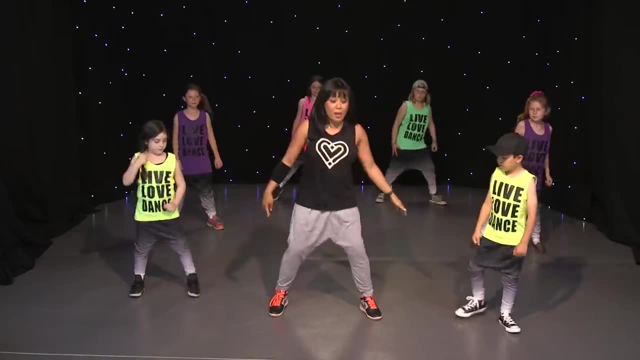 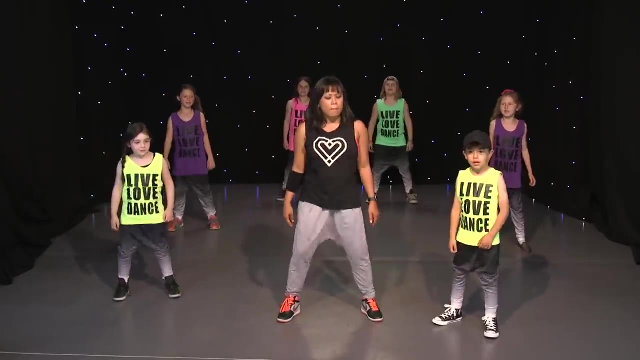 punch Again. Open, cross, open, cross, Punch, punch, punch, punch. Let's add some feet. You're going to take that right foot, You're going to step right foot behind, right foot behind, and then you're going to bounce it like you mean it, Like this: Bounce, bounce, bounce, bounce. 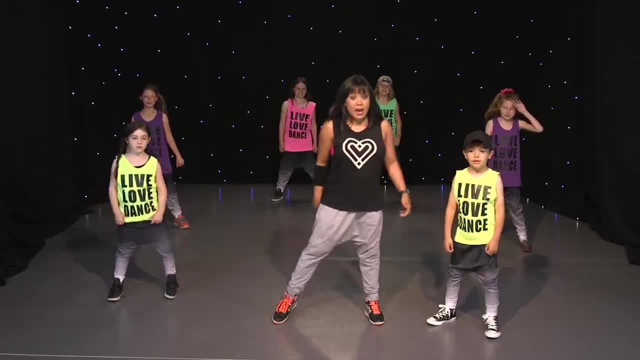 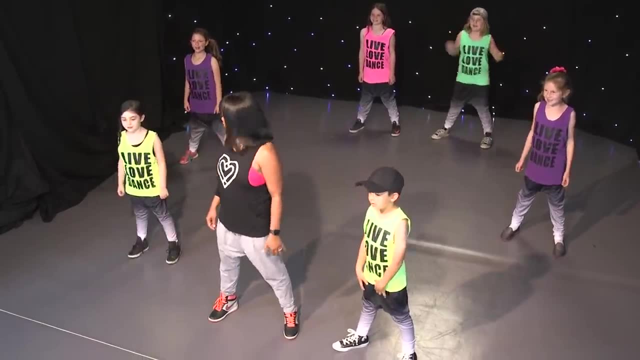 Don't they look so good? I mean, they're so good. right, Here we go, Step behind, step behind and bounce, bounce, bounce, bounce. Should we do it with some arms? Yeah, Why not? right, Here we go. Five, six, seven, eight. 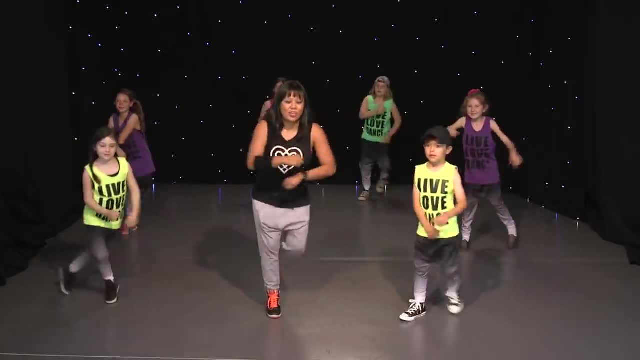 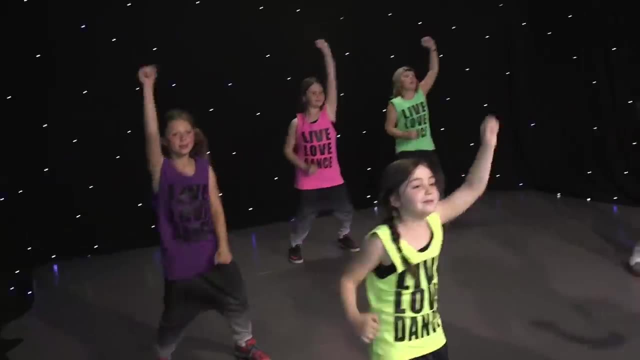 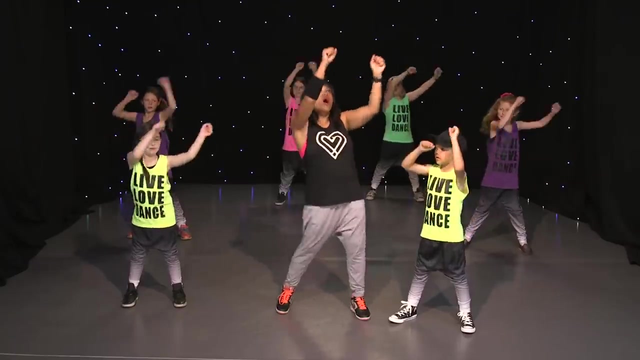 Six airplane arms. Go Airplane cross, airplane cross and bounce, bounce, bounce, bounce. Go Airplane cross, airplane cross and bounce bounce, bounce bounce. Last step, Super fun. You're going to punch all four corners like this: One, two, three, four and then you're. 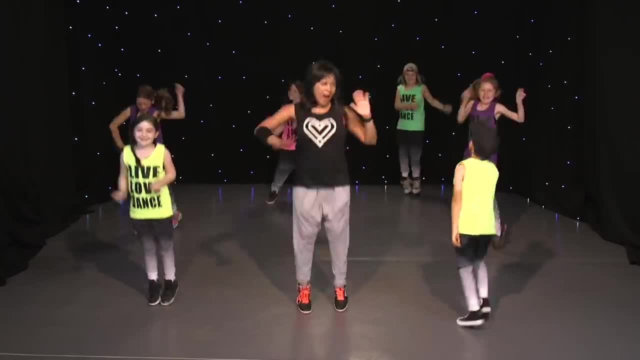 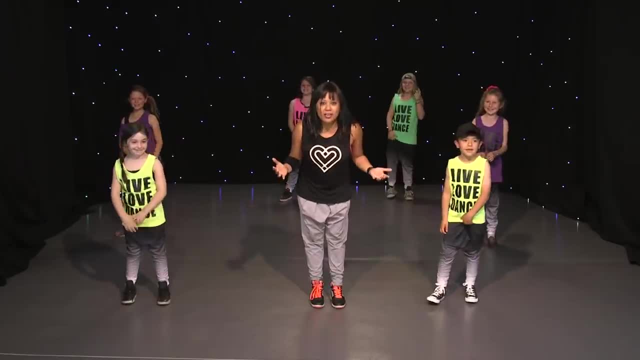 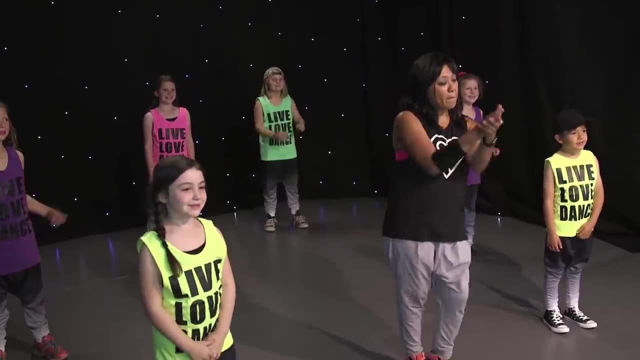 wow, wow, wow. What do you think? Easy enough, right? Should we try it with the music? I think so. Let's try it with the music. Here we go. All right, If you want to, you can add a little freestyle. 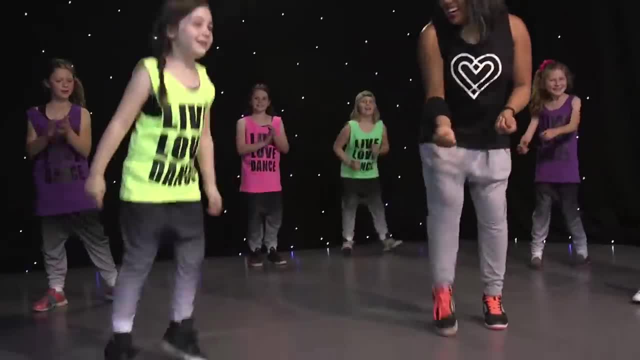 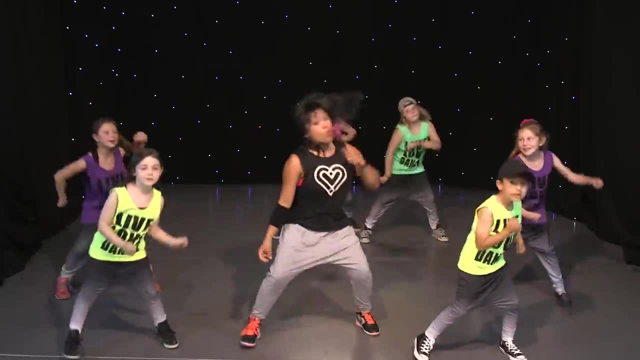 here. if you want to right Whatcha got Remy, Whatcha got Here, we go Right shoulder, Give it to me Ready, Go Hip, and one and two, three and four, and Oh yeah, oh yeah. 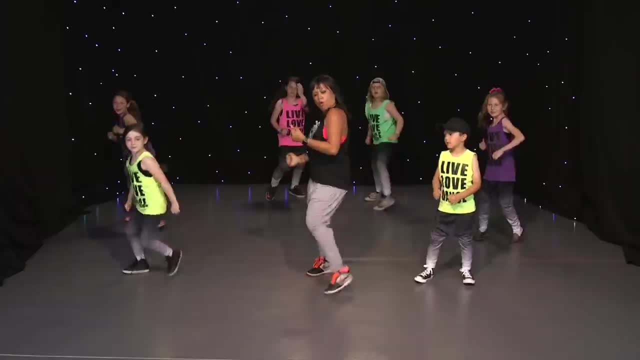 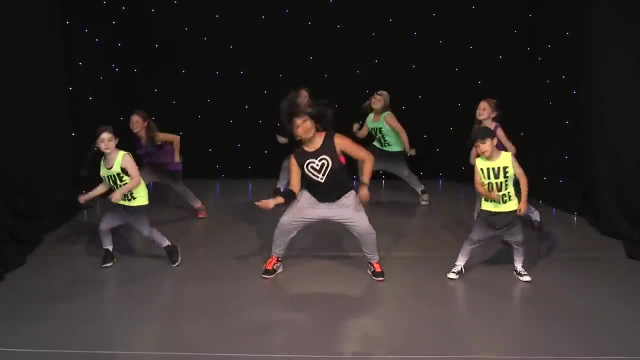 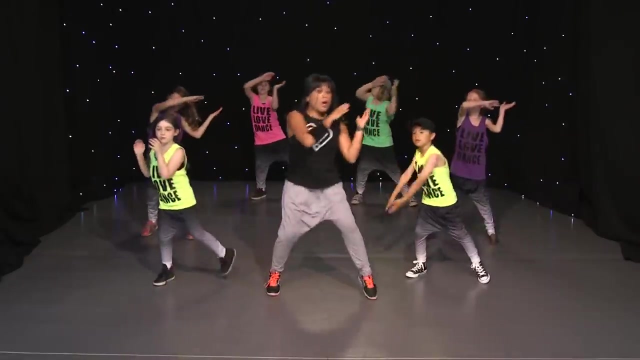 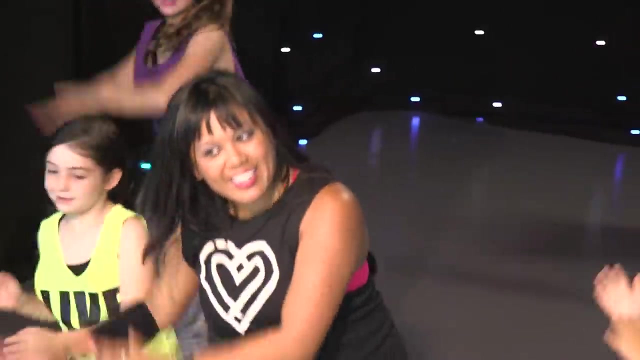 go Back back. Here we go, hup, oh yeah, oh yeah, take it back. woo, give me some rainbow arms. go chop it. like you mean it guys go chop it. oh, oh, oh, one more time go. alright, you ready for that airplane? let's do it. here we go. airplane arms. come on, hup, touch it. 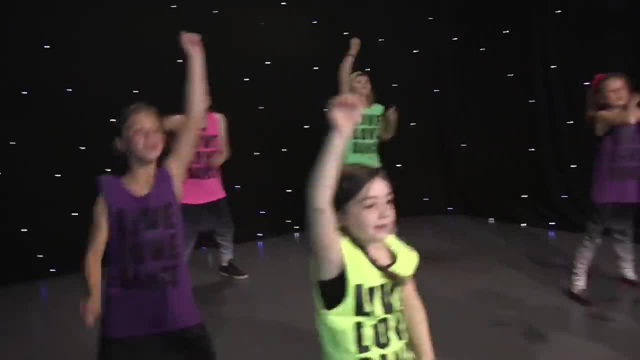 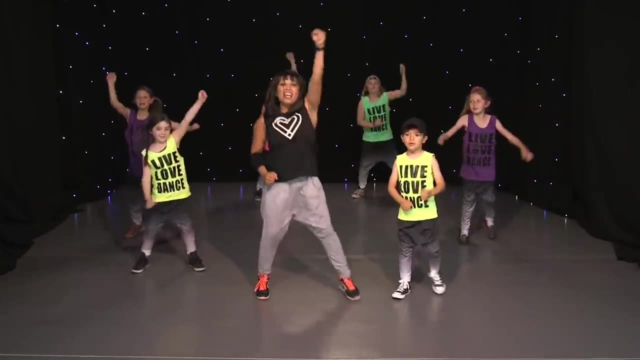 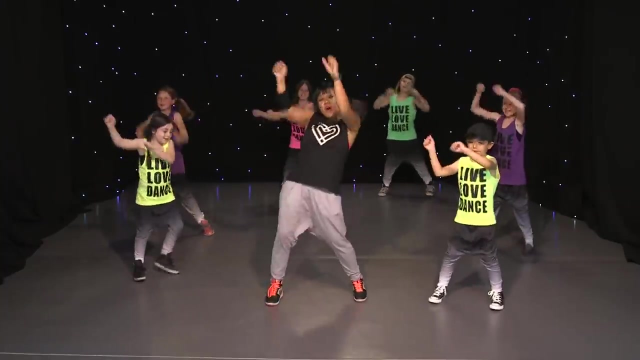 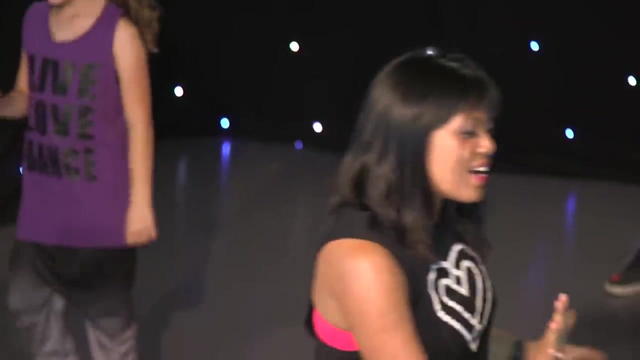 come on, alright, let's get crazy ready. four corners: go, get crazy, go woo. how'd we do? I think you did awesome. what do you think can we do it again one more time? can we do it again? 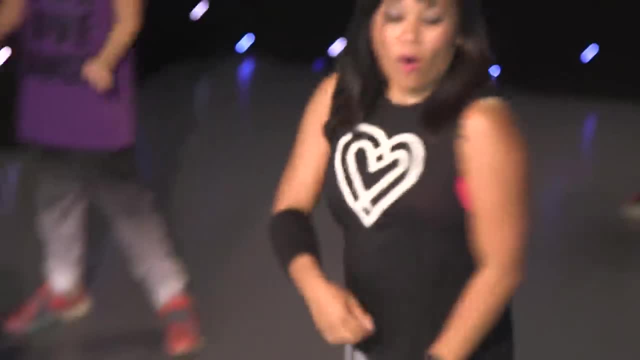 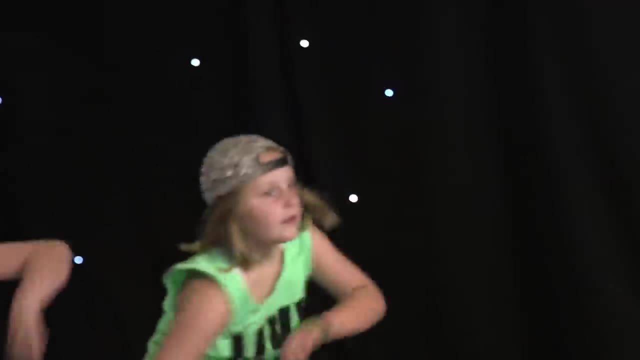 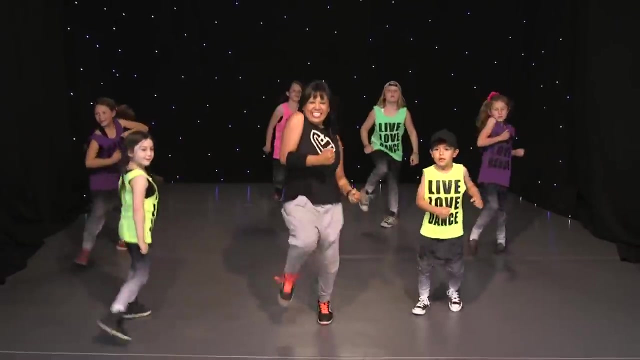 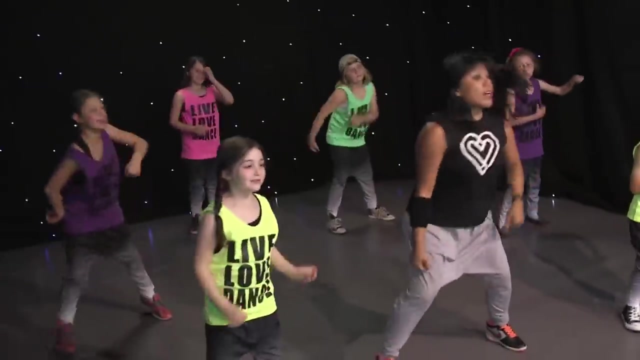 yes, I didn't hear you. yes, here we go. five, right shoulder five, six, here we go, snake it. oh yeah, woo again. come on, give me that rainbow, guys go chop it four times. 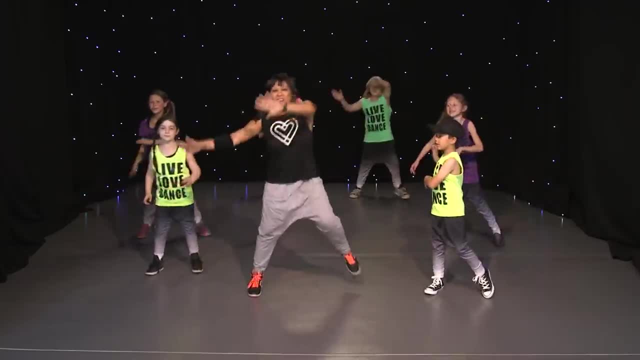 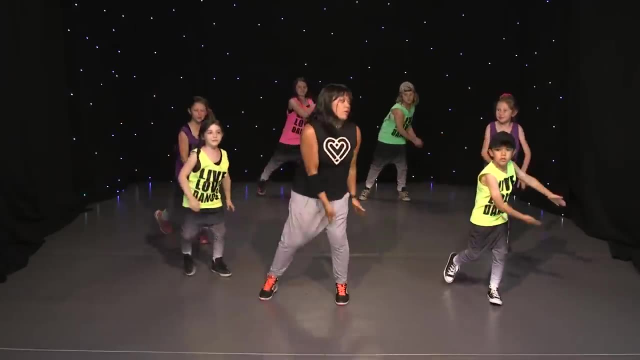 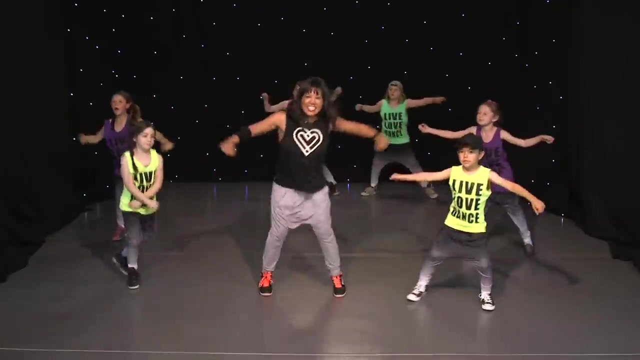 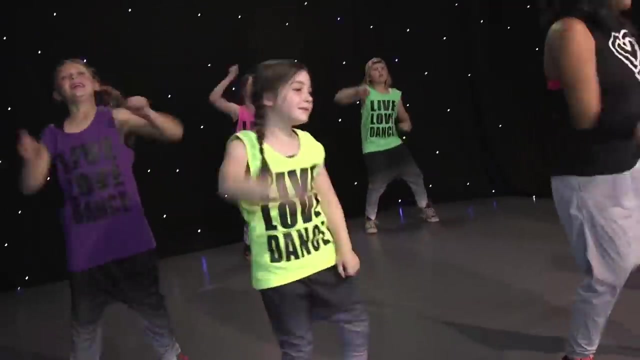 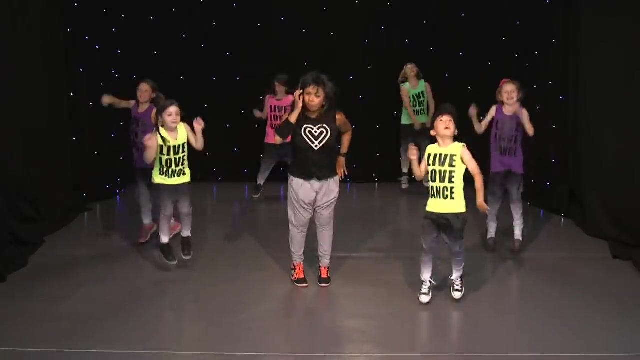 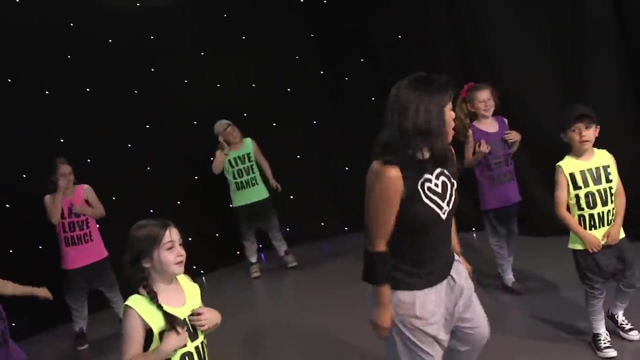 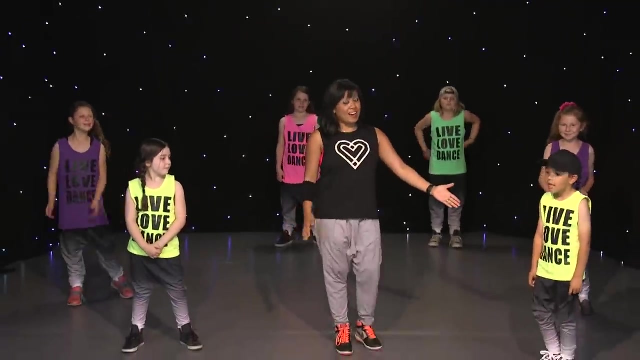 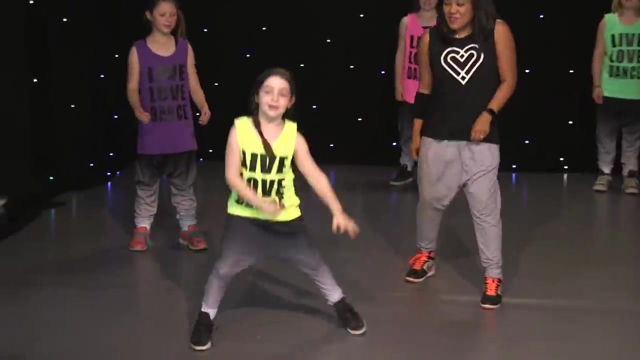 oh, oh, oh, one more time. go woo, chop it four times. here we go, airplane, let's go punch it. hup, give me two more woo. four corners ready. let me see you get crazy. woo, let me see you get crazy. yeah, how'd we do? I want you to meet my friends. they're so special to me. do you want to meet my friends? alright, well, this is Jonah. go, Jonah. this is my friend Randy woo. this is Emma. 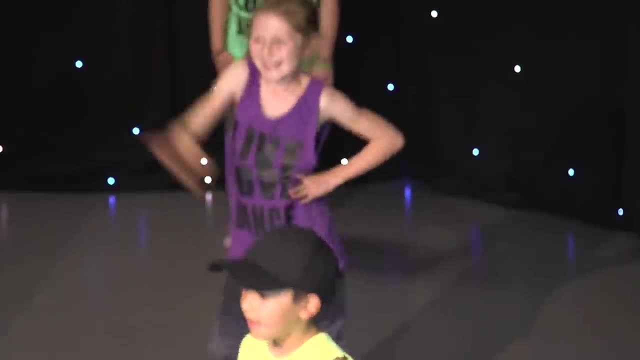 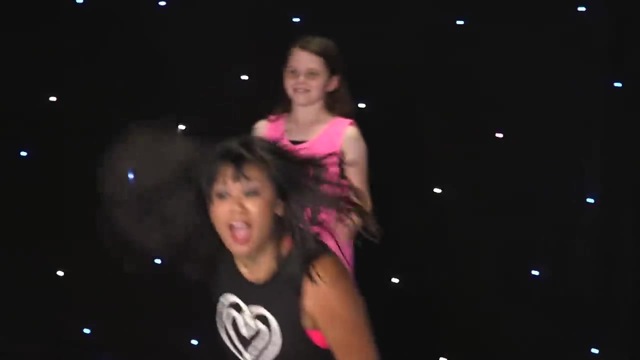 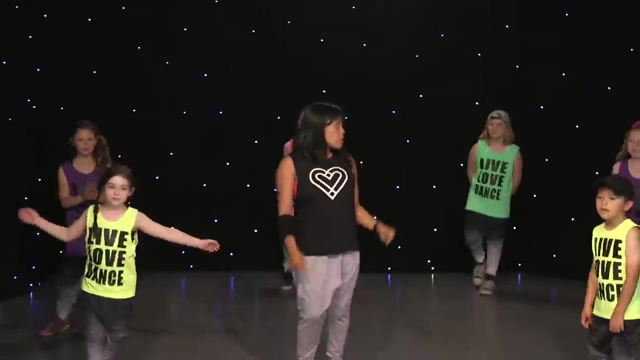 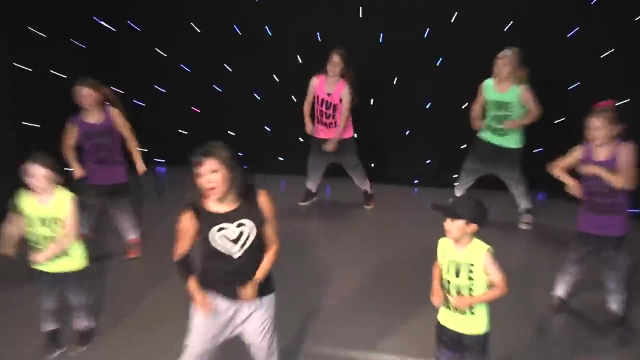 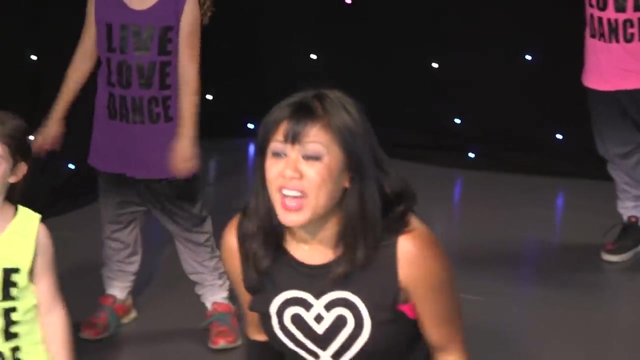 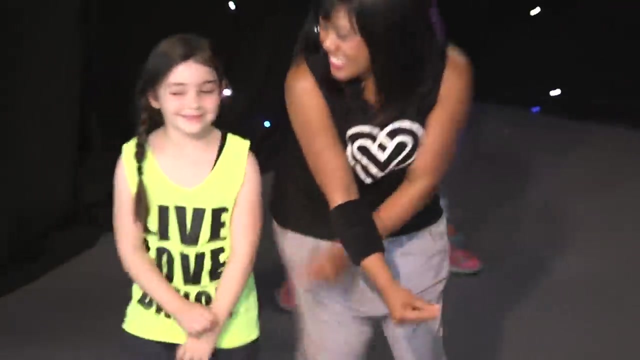 nice. this is a lot. this is my friend, Tanya. this is Emily. yeah, you ready? give me those four corners, let's go crazy. woo, thank you for dancing with us. you guys, we'll see you next time. you guys have a good one. woo, break it down, go Jonah, go Jonah.